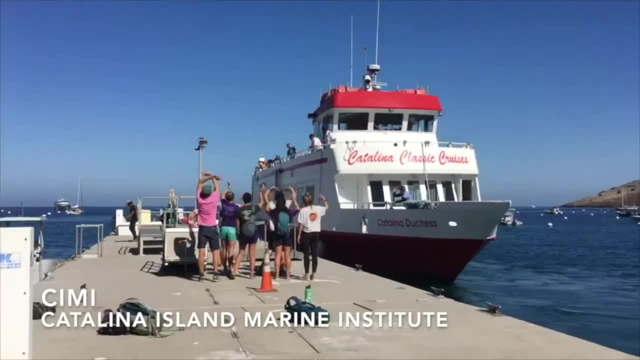 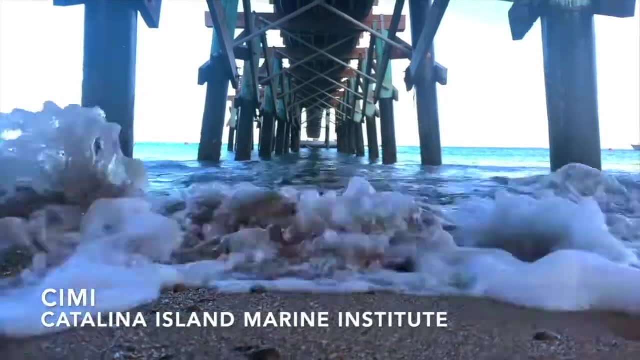 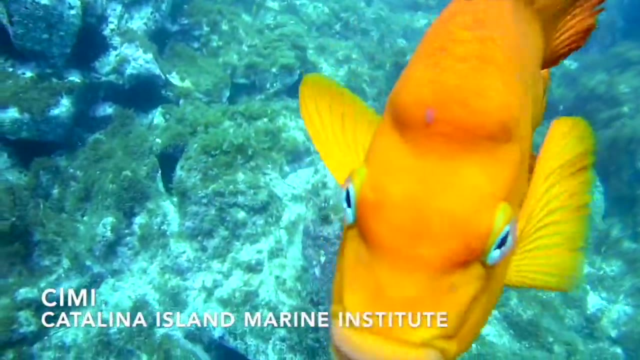 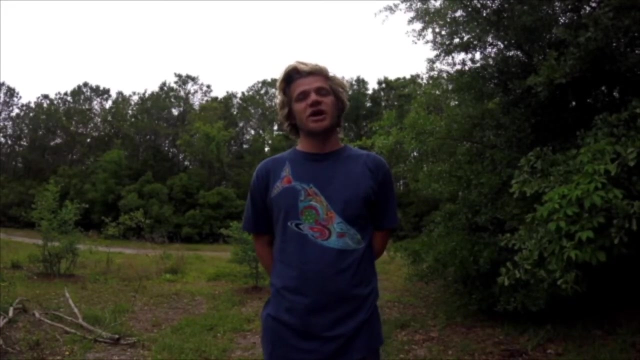 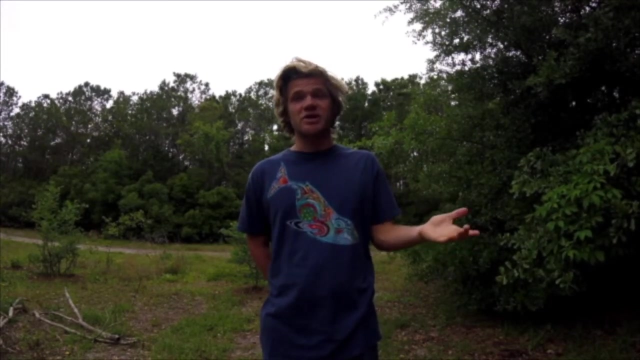 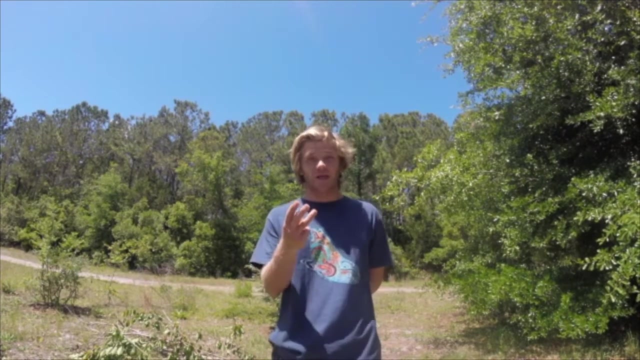 Hey everyone, I'm Jake Ciesielski and I'm an instructor at Fox Landing and I'm going to teach you about physical oceanography, specifically how waves are created and how they move. Before we do this experiment involving the line, we are going to break it down into three steps. 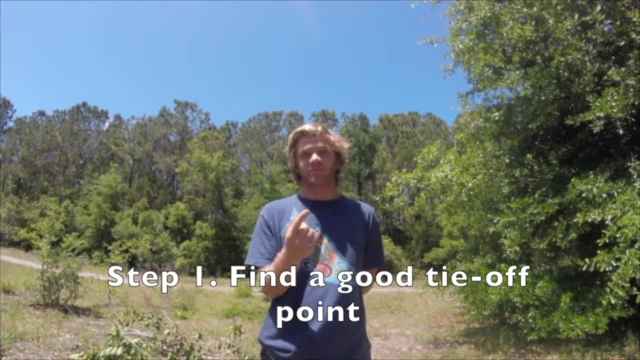 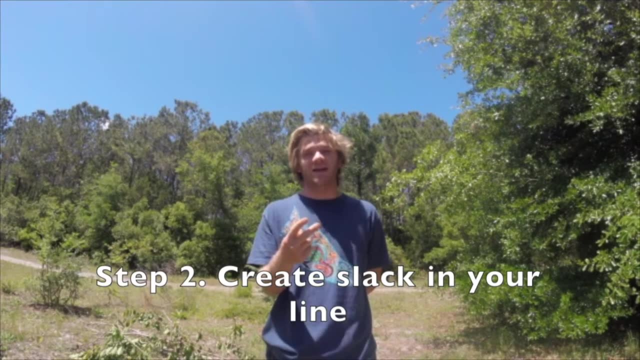 The first is going to be your tie-off point. Your tie-off point is going to be your shore and where the water is going to be breaking. The second is going to be the slack in your line, which will signify as the energy moving through the ocean. Lastly, you're going to be holding. 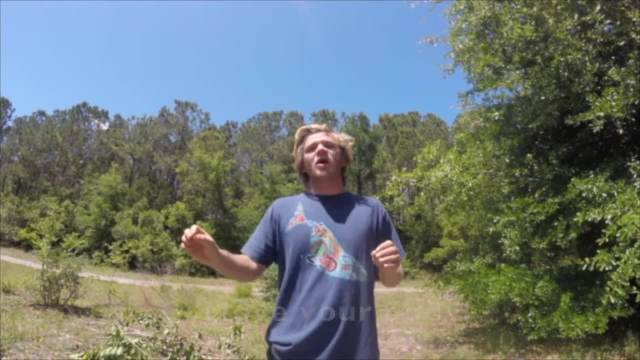 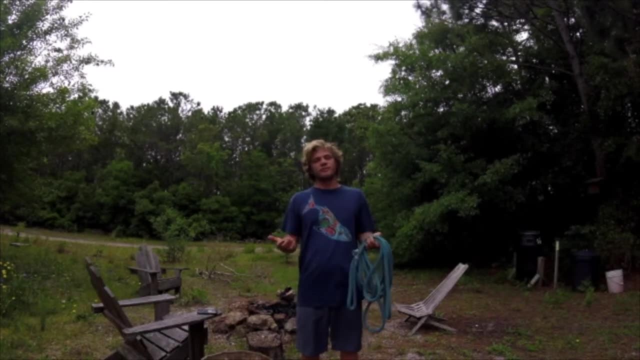 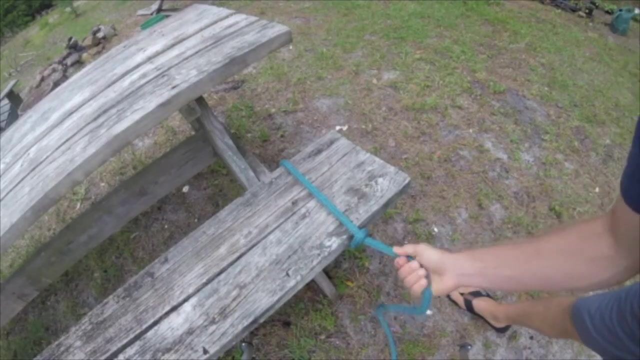 the line and whipping the line simulating the transfer of energy through the water. For this first experiment, we are going to show how waves move, So the only materials that you're going to be using is a line. So the first step is you're going to be tying off this line to a 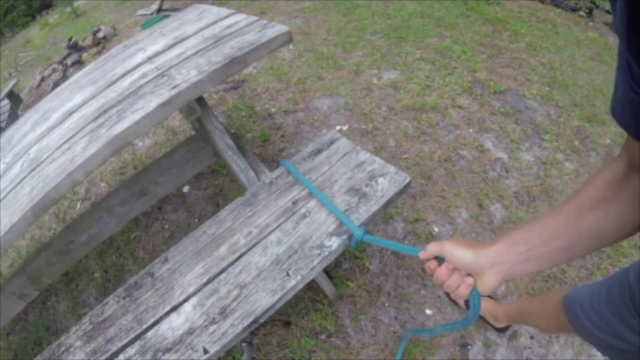 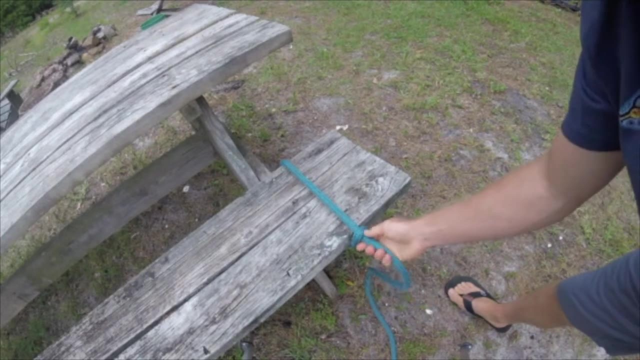 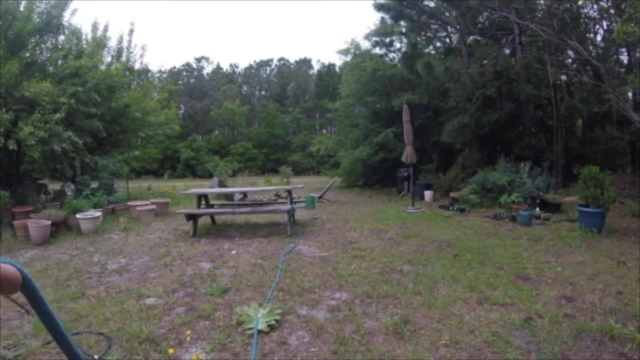 point. It can either be a table, it could be a post, Just make sure that the point is sturdy. Remember this is going to signify as your beach or your spot, which is where the wave is going to be breaking at. The second step is to walk backwards with your line holding it and to still leave a little bit of slack. 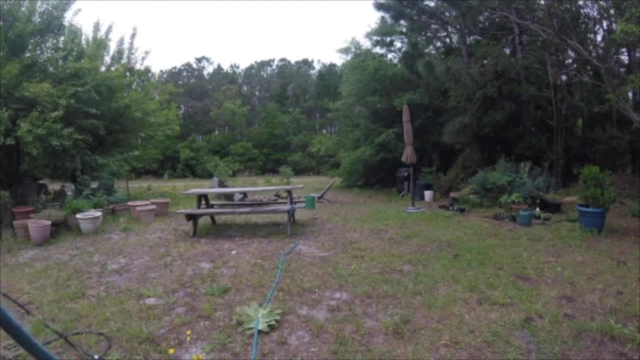 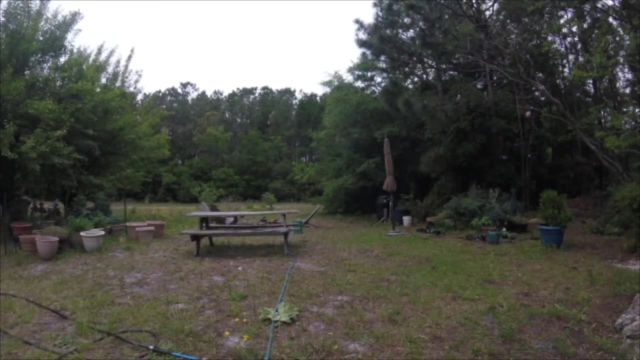 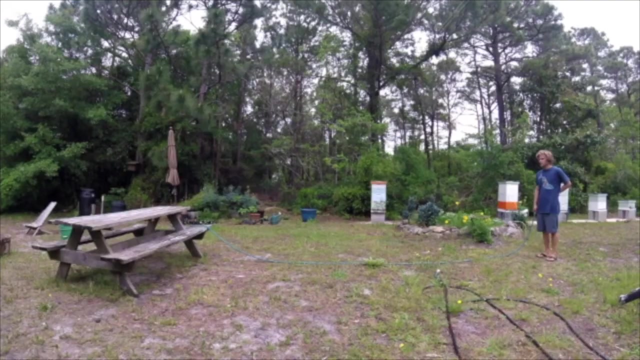 or just making sure that the line is still on the ground. And third and last step is you're going to be creating the experiment. So all you're going to be doing is making a whipping motion with the line like this, And this is how it will look like. 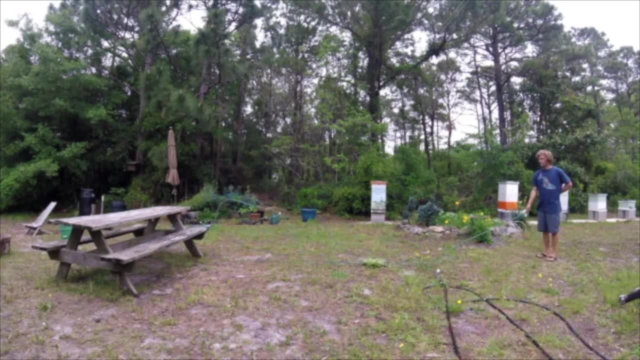 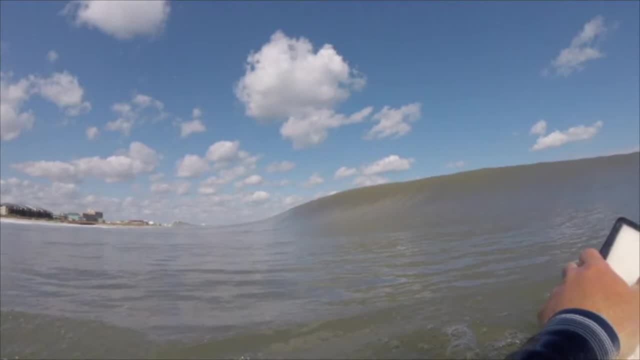 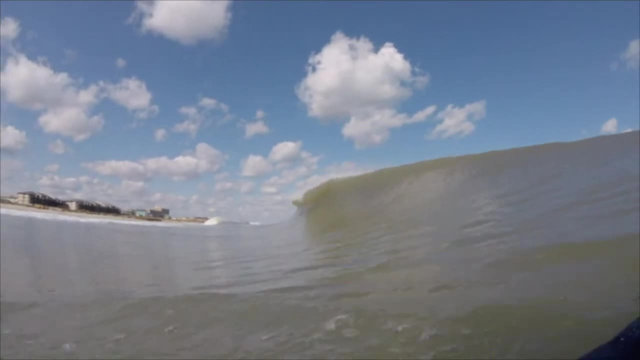 OK, so we're going to do one more time. Let's head to the event floor And in between the waves, we're going to be taking a look at the time of the experiment. Now the time is 11 o'clock. 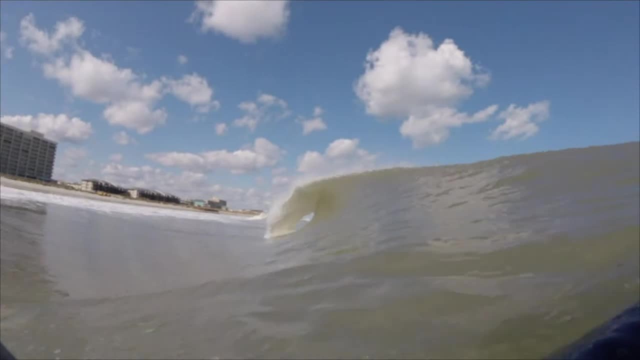 We're going to start with the time at which we're going to see the future of the ocean. So let's start with the time at which we are going to see the future of the ocean. the present moment Time is qualquer. It's going to be 5,, 6,, 8,, 10,, 11, 11, 1, 2, 3, 2, 3, 2, 3, 3, 2, 2, 3, 2, 3, 2, 1, 2, 2, 2, 1.. 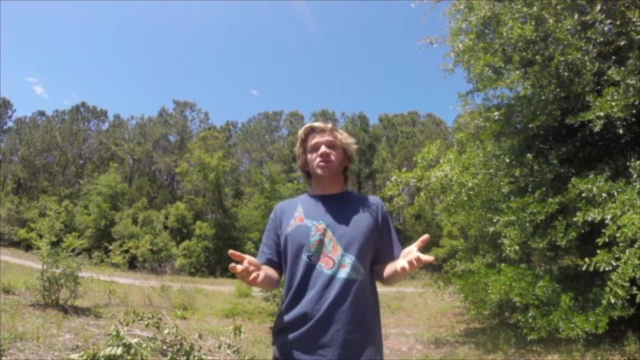 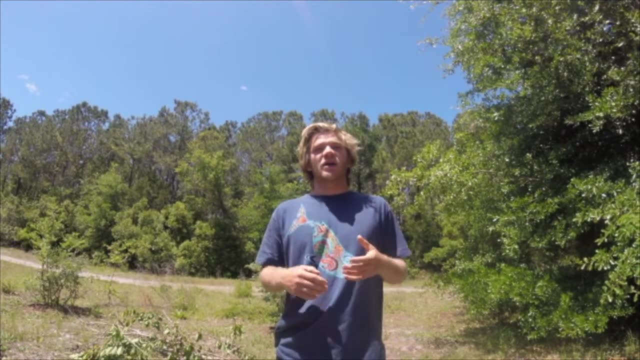 Now let's start with the time. Let's look at the time at which we are going to see the future of the ocean. ocean but energy. The ocean transfers this energy like a medium, similar to how sound waves travel through the air. That is why, in physical oceanography, we call ocean waves. 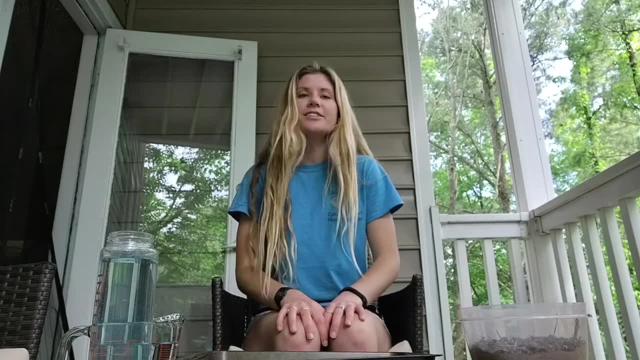 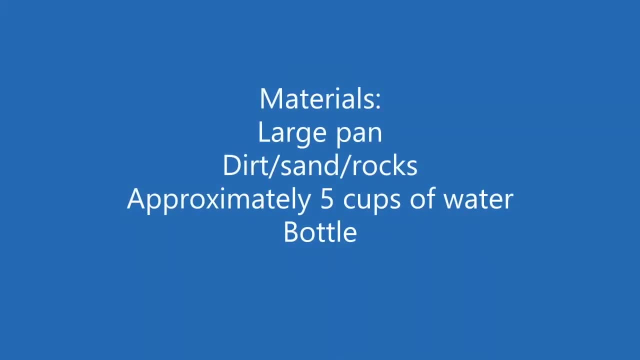 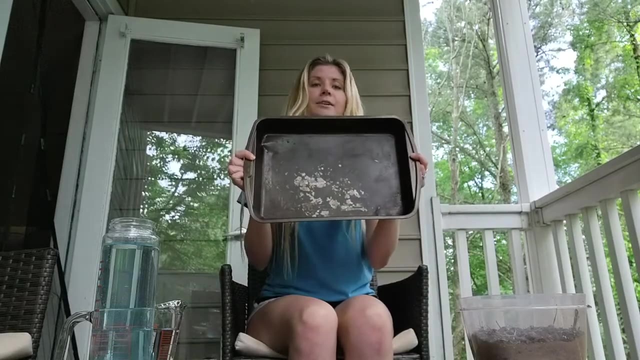 medium waves. Thanks, Jake. Now that we understand waves a little better, let's see what happens when they keep repeatedly crashing on shore. For this experiment, I used a 10 by 14 inch pan. It works better if it's glass, but this. 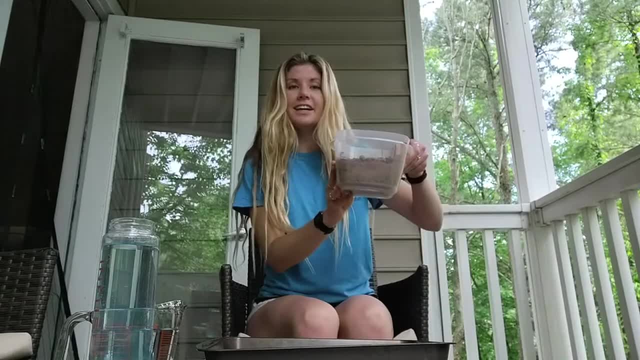 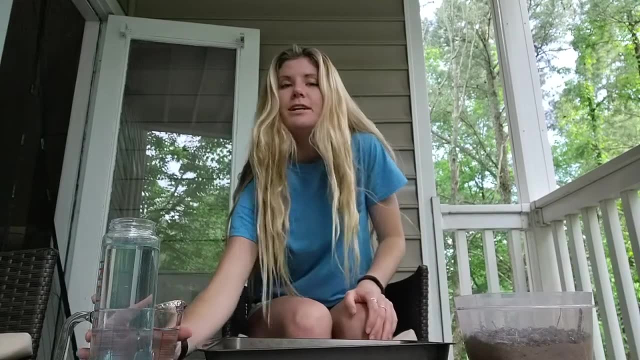 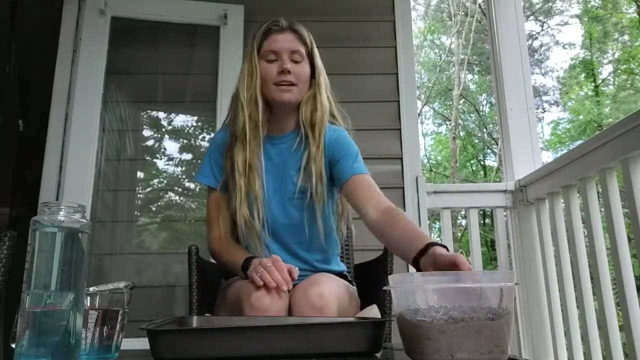 is all I have. I went outside and collected some dirt. Works better if you have sand, but collect whatever's outside your house And grab some water. I colored mine blue so it looks just like the ocean. The first step is to pour your dirt or sand into the pan. 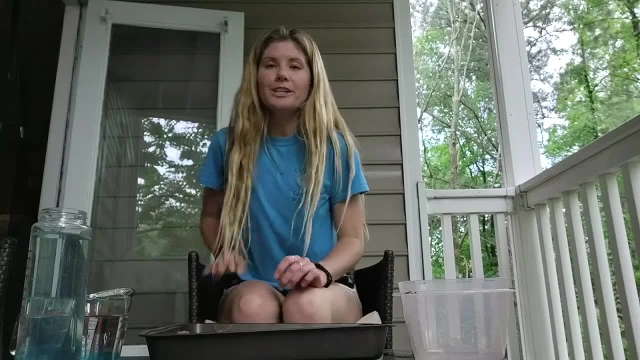 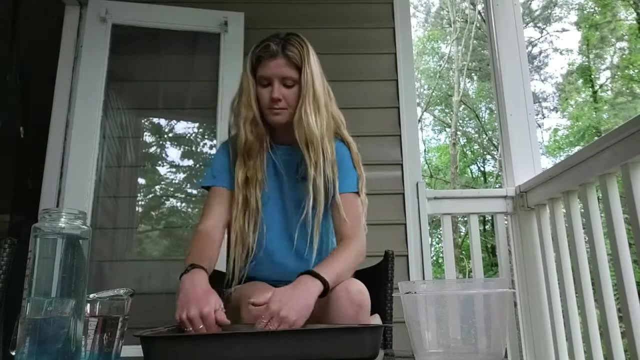 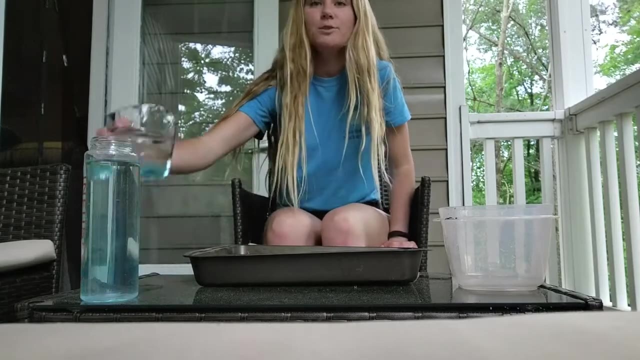 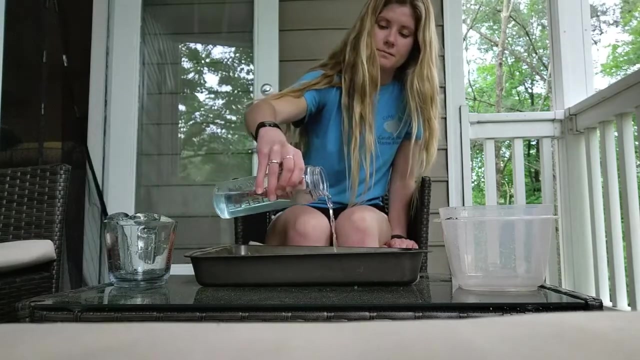 Okay, Once you pour in your dirt, shape it just like a shoreline. Now we can add in our ocean water, Just pour this, on the opposite side of your sand, Once you pour in your water, you want it to be about halfway up the slope that you're. 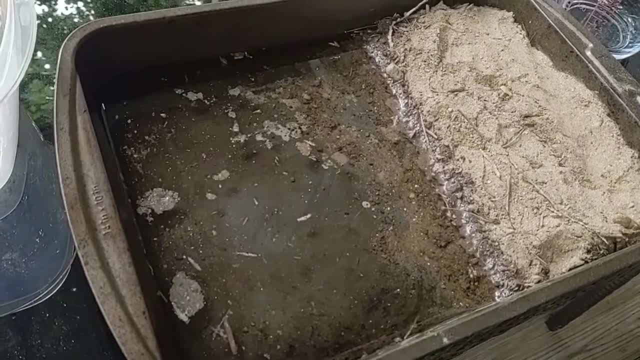 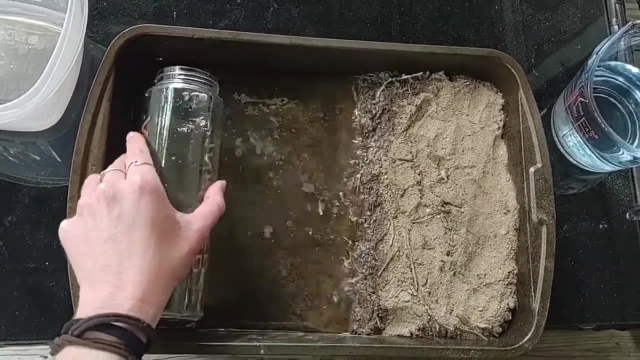 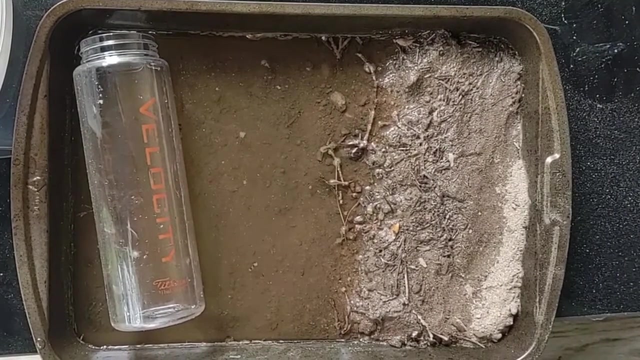 using your dirt and sand like this: Just move the bottle up and down to create waves. After about a minute of waves, our shoreline has changed. This change is caused by erosion, which is the wearing away of the sand, shells and rocks all along the shoreline. 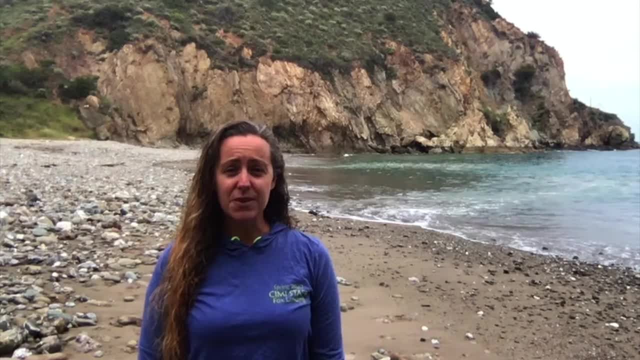 Now that we learned a little from Jake and Abby, let's recap: Waves are the transfer of energy to the ocean. Let's recap: Waves are the transfer of energy to the ocean. So when we have a very, very high temperature, we're actually losing a lot of air. 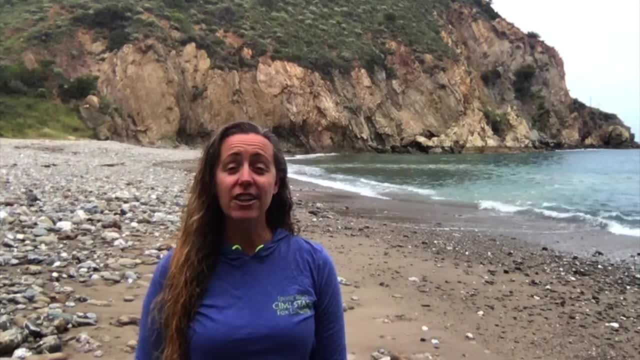 When you have high temperature, we are losing a lot of air. When we have a very, very low temperature, we're losing a lot of air through water, sometimes traveling as far as hundreds of miles. We talked about what happens when those waves meet the beach and how they play a role in. 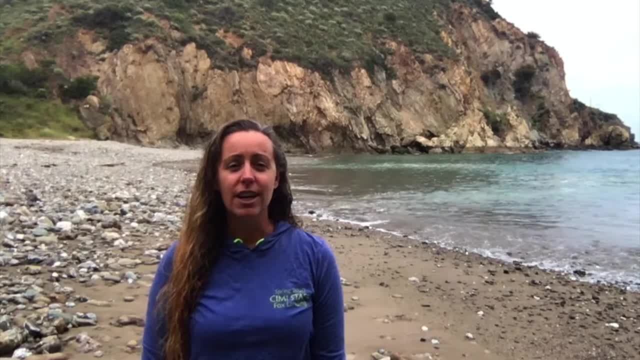 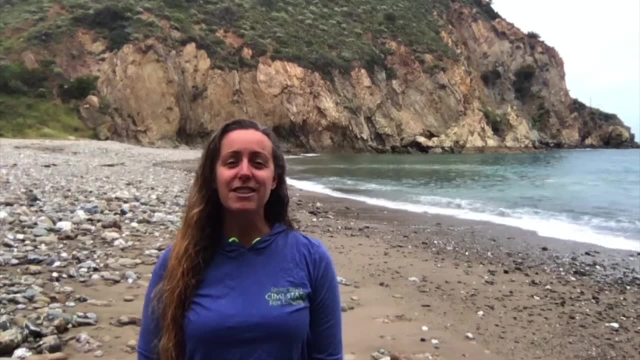 shaping our coastlines through the natural process of erosion. Try these experiments at home and explore what happens when you use thicker or thinner ropes, make bigger or smaller waves, and using different substances like sand and rock. Thanks for watching.